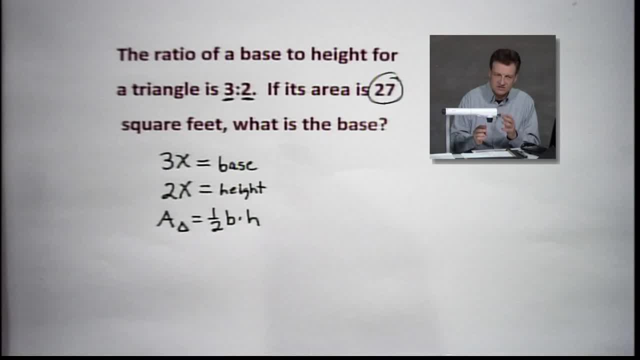 and then we hope that we have enough information that we can solve the rest of the equation and find our missing lengths. okay, In this case, missing lengths- Ah, a little play on words there. all right, Let's see what we've got going here. I know the area We're told. 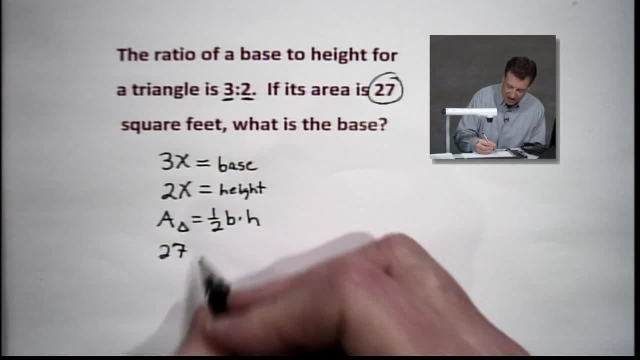 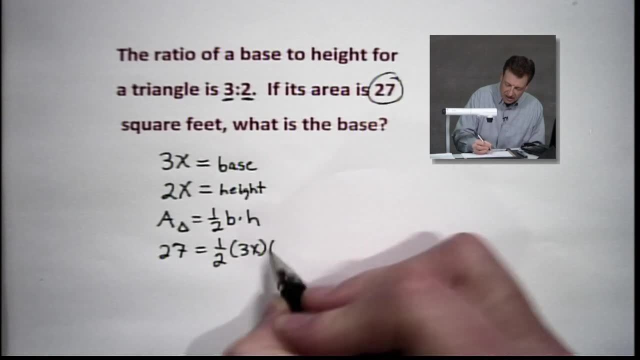 it's 27.. It's, of course, in square feet. We'll put our 27 there, Equaling to one-half. my base is now 3x And my height is 2x. That comes from that ratio. That comes from putting the x next. 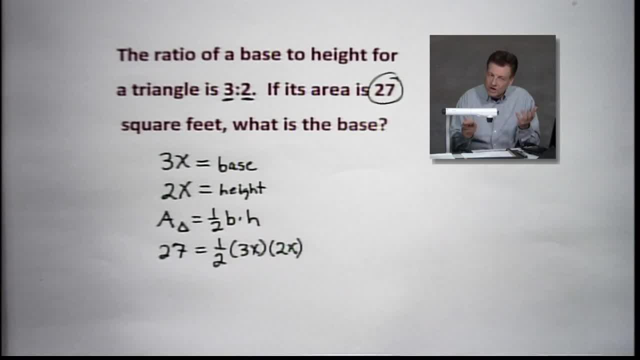 to those. That's 3 times x, remember, and 2 times x. So we're still in the money here, all right. Now here's where my students sometimes go astray. We look at this one-half and we. 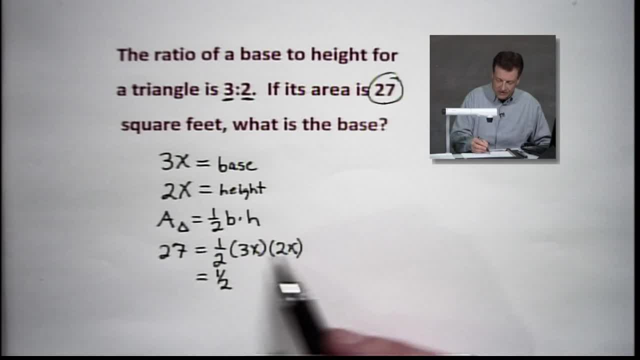 notice: 3x times 2x And they get all excited. And 3 times 2 is 6.. Mm-hmm. And they say x times x is x, It is not x, It is x squared. So be careful on that. okay, Be careful on that. And we still keep our 27 rocking and 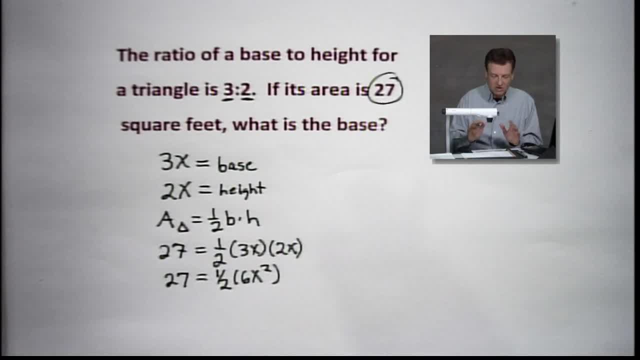 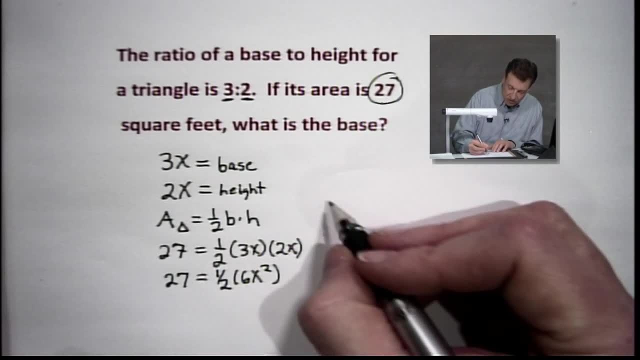 rolling right over there. all right, Now you've got a couple of angles to go on this. Since half and 6, half is and 6 is even and half of 6, we can figure out, I'm gonna go ahead and say we'll move right over here. 27 is equal to. we'll bring it right up here. 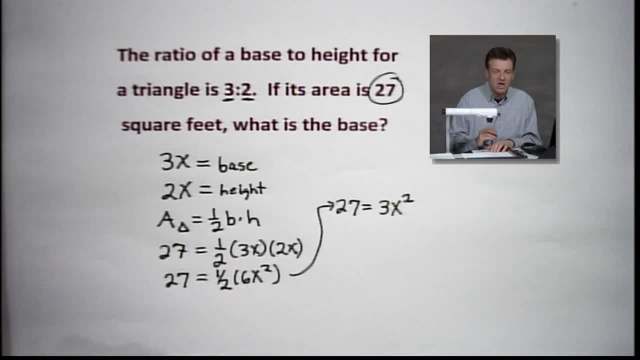 and it's gonna be 3x squared. You say, well, Ernie, that looks nice, It does, because we're getting down to a point where we're gonna get x by itself. It's gonna be rather simple and rather easy to do. The 3 is hooked into this x squared by a multiplication. so let's. 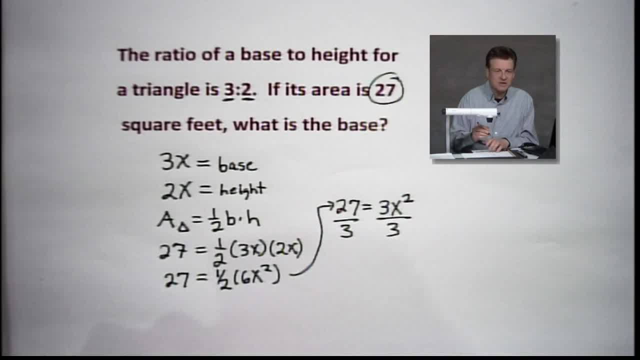 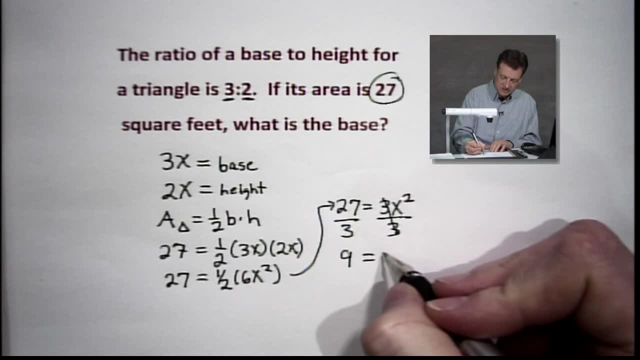 divide it out, take it out and 3 goes into 27,. a nice number, a nice number. It's a perfect square. So let's go with 9, and then our 3s take care of themselves, and we've got x squared. 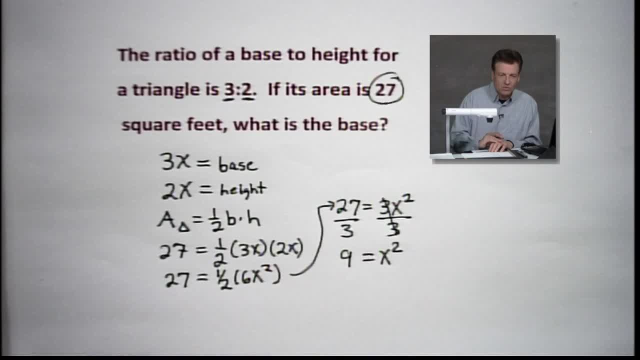 by itself. Boy, talk about the 3s, because guess what? We're gonna square root this 9, and we're gonna square root x squared, and that's gonna leave us with x equals well, 3.. And you say: oh, the answer's 3.. No, no, no, no, no. we gotta come back up here, Gotta.